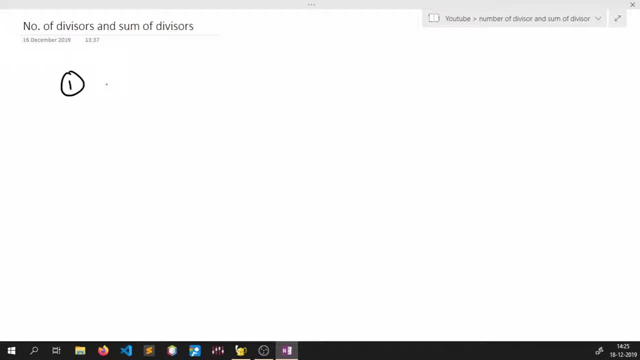 so let's clear why we are adding one first. so suppose we have a number such that it has only one prime factor, which is p, p 1, e to the power 1. so if there is only one power here, we know that this number will be one. then p 1, p 1 square, and up to p, whatever that power is, e 1- okay, we. 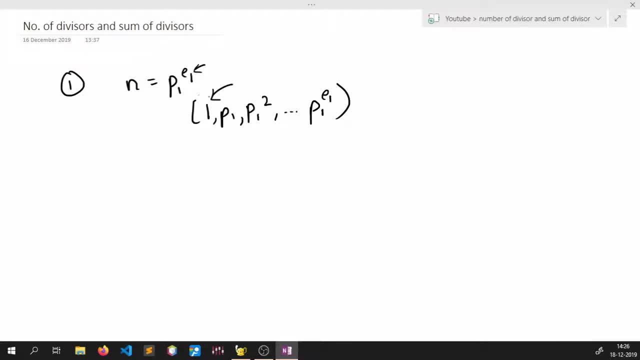 know this because we will take this one and multiply with every power of this thing. so we'll multiply it with this, with this. so the reason for adding one is we are taking one with every prime number, because one is always a factor of a number. if the number is even prime or anything, one is. 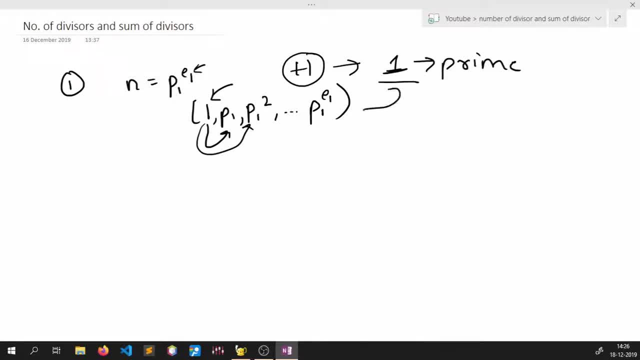 always a factor. so that's why we are taking it separately here and we are adding one to this power. so this was the logic for one and for multiplication the logic was: uh, let's take that number again- p, e1, and let's say this time we have two means, two prime factors, and its power is e2. 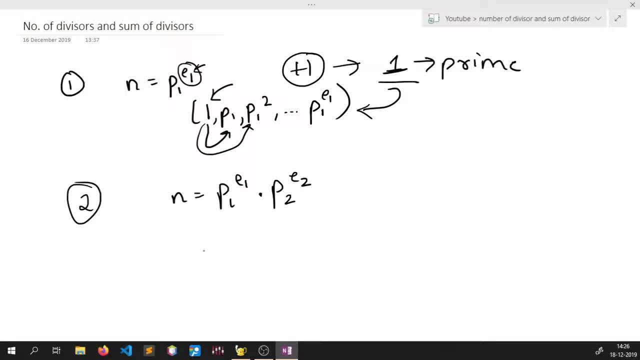 so what do i mean by this is: first we can make a table like this: so let us take one here and let me take p2 here. then i will take p2 square here and up till p to the power e2, okay. and then i will take p1 here. then i can take p1 square here and you know it will go up till p1. 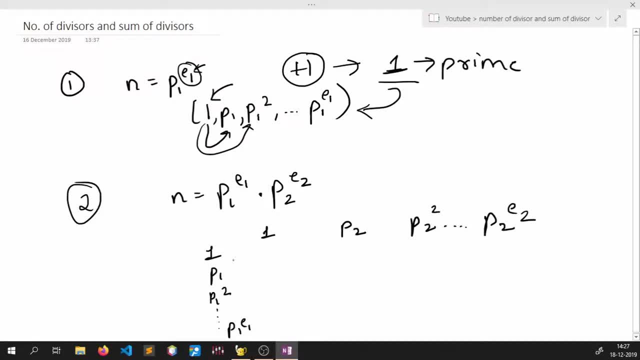 to the power e1. okay, so one and one. so one into one will be one, one into p2 will be p2 and one into p2 square will be p2 square and here we will have p1 square. then we will have p1 square, p2. 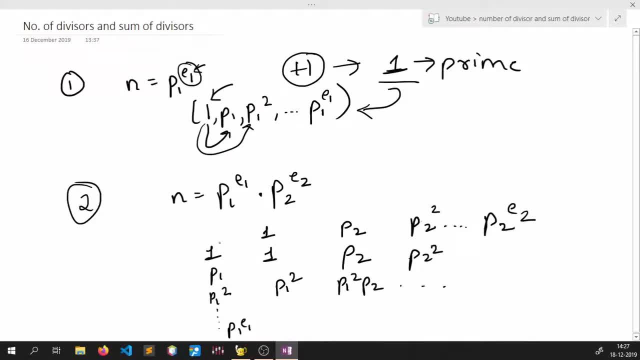 and so on. so what we are doing is we are taking all the combinations of these first prime number with all the other prime number we are getting in factorization. so we are taking all these combinations. so because we are taking combination, we are multiplying them. we are multiplying their power by adding one and the reason for adding one. 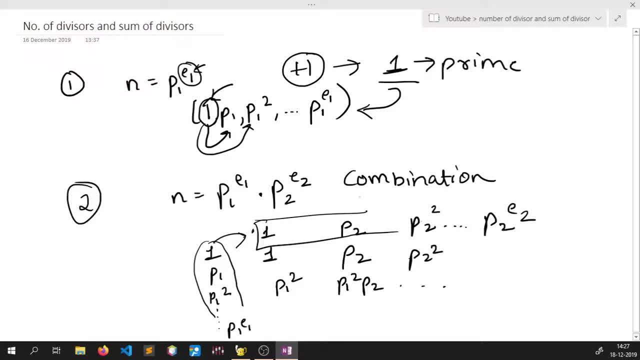 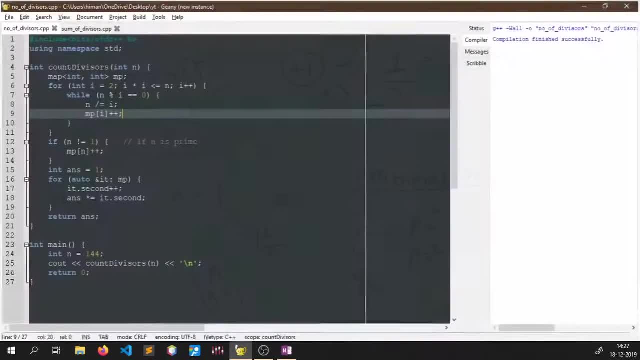 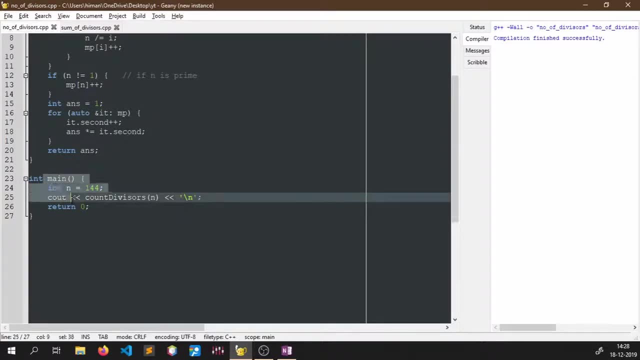 i have told, because of this, one extra one and the multiplication is because of combination. okay, so now let us look at the code of this. let me open it. so this is number of divisor, the code for number of divisor. so let's start with main. so here is our main. uh, we have taken 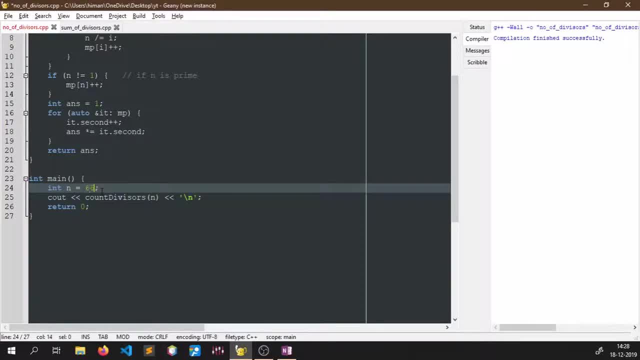 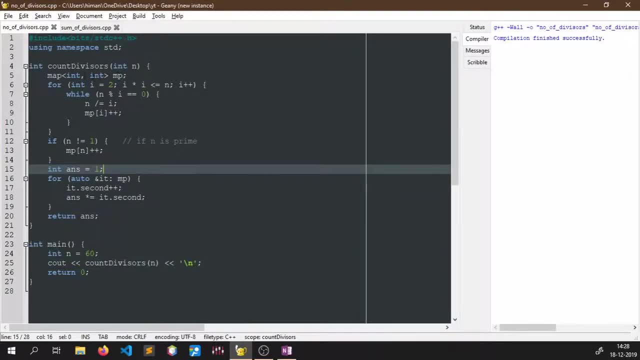 a number like 144, let me change it to 60, which we took in our example. okay, so we have a function- count divisors- which will count the number of divisors. so we have created first a map map. and why we have created a map is i'll explain it to you on the go. 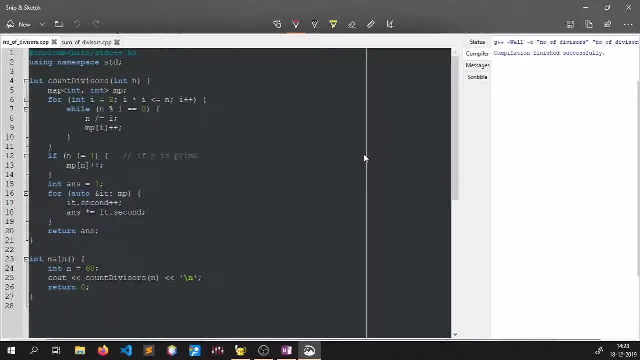 let me have a snip of this thing and i'll explain it here. so we are taking a map mp here, and then we are iterating. so this is the loop for finding primes, that so we will start from 2 and we will go till square root of. 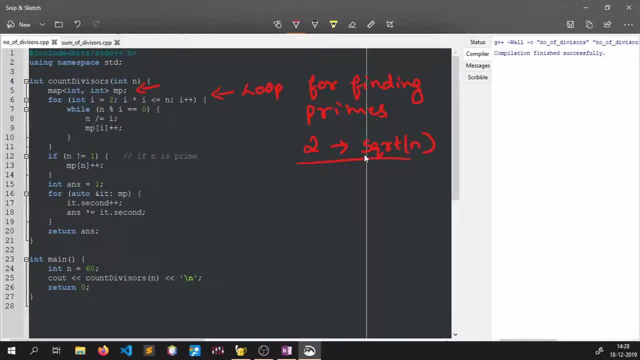 the number n, which is an efficient way of finding a prime number. so if a number is dividing it, that means that is a prime factor of it. so what we will do is we will keep on dividing to calculate the power. so let's say we have four, so we have a two as a prime factor of this total power. two so 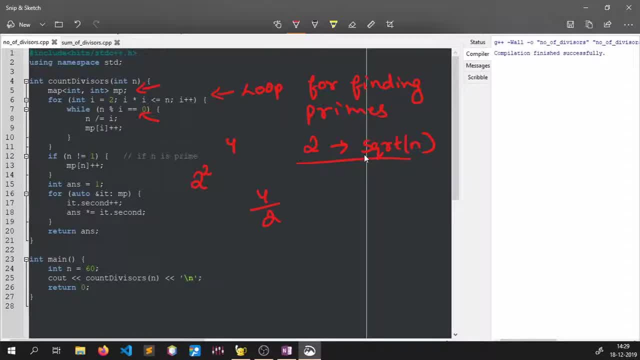 we will divide it by two and inside the map of two, first it was two comma zero. then we will divide it once, so it will become two, and here we are adding mp of what i. i is two. so we two, this two, we are doing a plus plus. so what will it make? is it will get converted into two and then one. 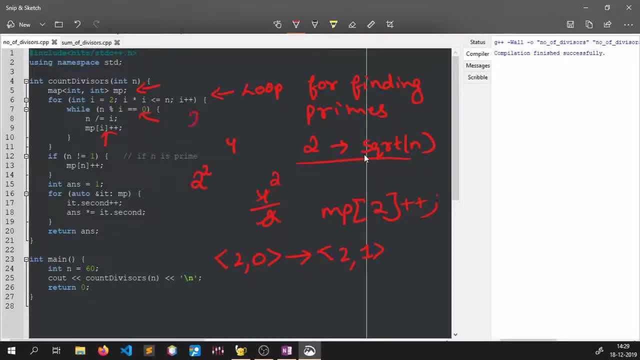 then again we have y loop, so we know that two more two is equal to zero. so we'll divide it again, so it will become two by two, and then we will have one here and mp plus plus again, so it will get converted into uh, two comma two. this will be the pair inside the map, so this: 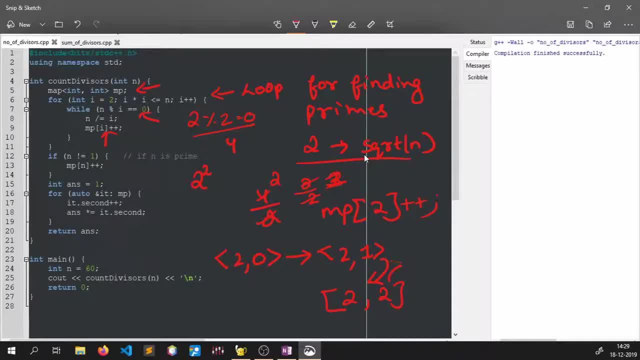 will be key and this will be uh, this will be value. so this value will represent e, one e, and this key will represent p. so as we write the form p to the power e, so similarly there will be multiple keys. so we will name it as p1. 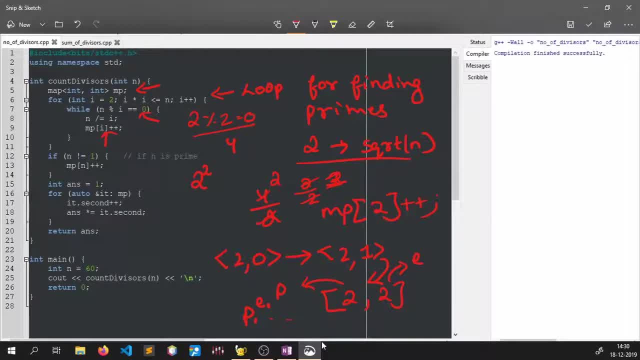 to the power e1, and so on, p to the power p2 and further. so this was our logic and, at last, what we are doing is: let me sorry, let me erase this thing, okay, let me erase it completely, okay. so, after finding this prime numbers up to layer, now we are checking if and 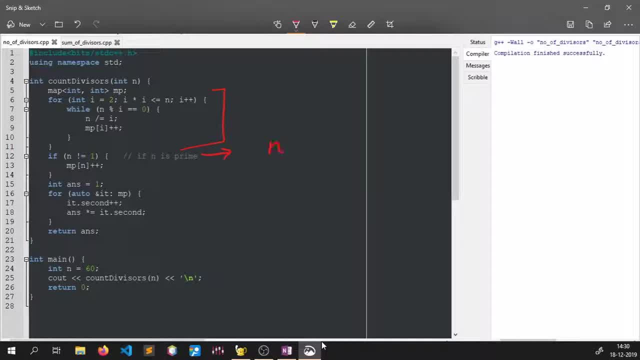 itself is a prime. so if itself is a prime, we have to count that power, that n, to the power, something okay. so we are adding mp to the n plus plus, that is, the number itself is a prime factor of itself. so if we suppose take 13, so what we will get is 13 to the power of 1, because 13 is 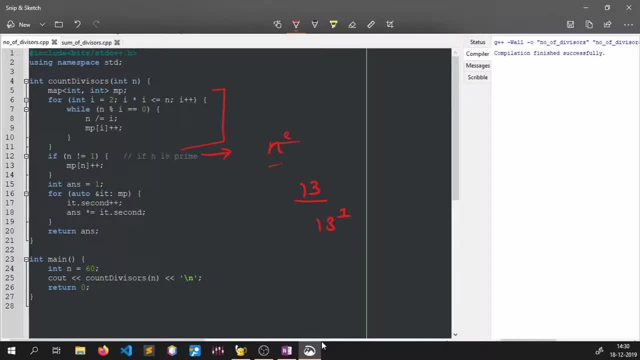 the prime number. so we are adding mp n plus plus, so it will be 13 and 1. okay, now what is this slope doing is we are doing the multiple work. so first we are adding 1 to every power. that was our e 1 plus 1. this is: 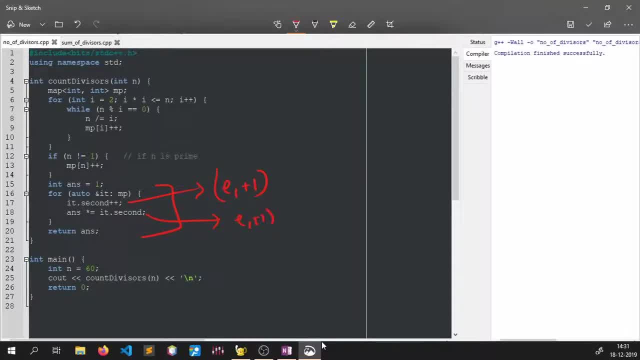 adding 1 and this is multiplying. so e 1 plus 1 is getting multiplied with its previous result. or we can say e 2 plus 1, this is n 2, and this further goes on till we reach the end of the map. okay, so we are multiplying it and the answer we 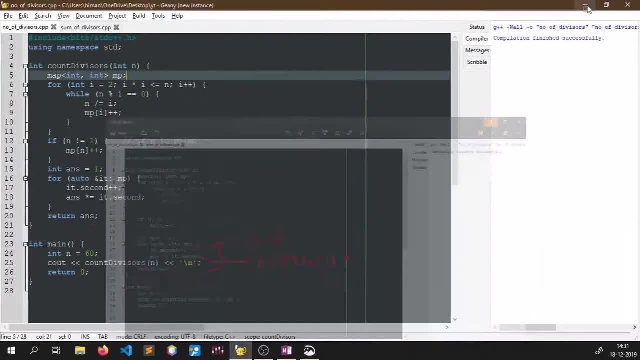 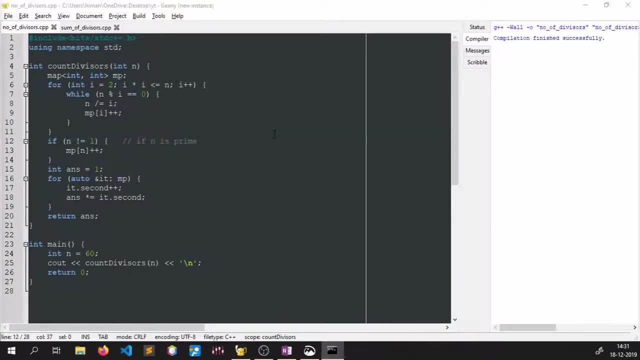 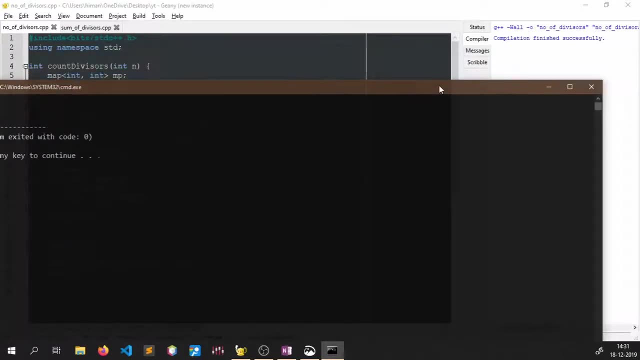 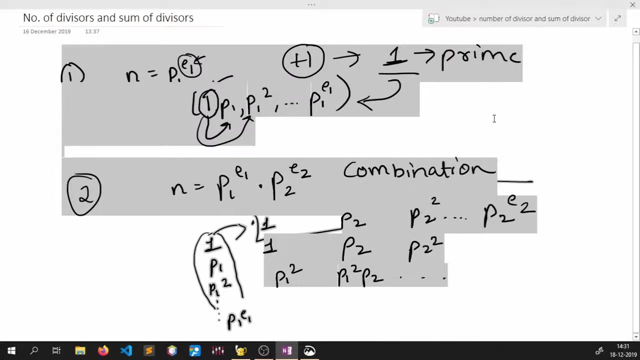 are returning here. let me run this code and see if it works fine or not. let me compile it. okay, so compilation successful. now I'll run it and let me show you the output. so the output here is tos we saw here. let me open this. okay, so for 60, we show. yeah, for 60, we have done that. it was true to the power. 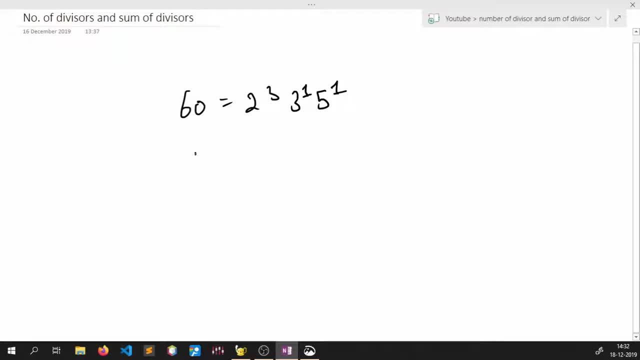 3, 3 to the power 1 and 5 to the power 1, and we will get an answer like 2, 3 plus 1, 1 into 1 plus 1 into 1 plus 1, so it will be 4 into 2. 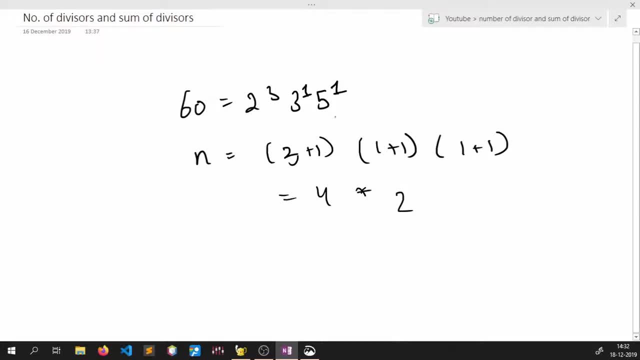 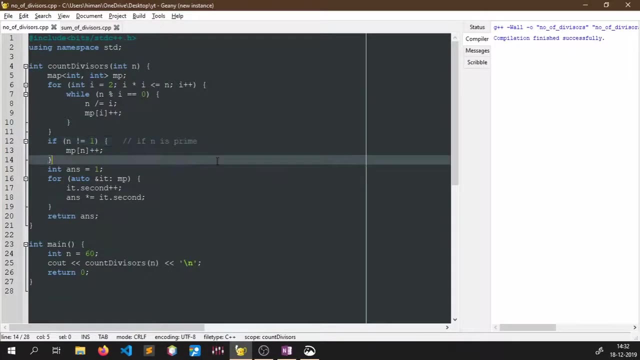 okay, it will be 2. oh, sorry for this mistake, it will be 2. yeah, so we are getting 3 into 2 and then again into 2, so it will be 12, and the answer we are getting is 12 itself here. so i rent and the answer is 12. so this is the code. i'll give the link in the description for: 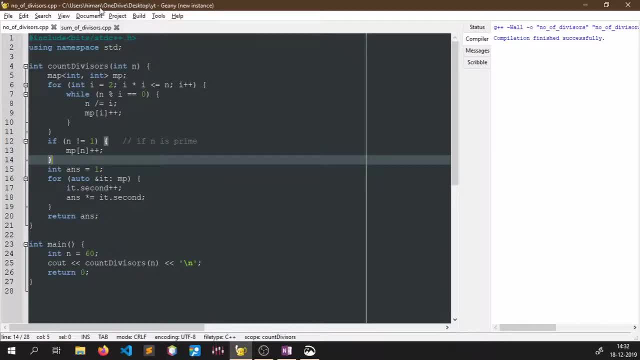 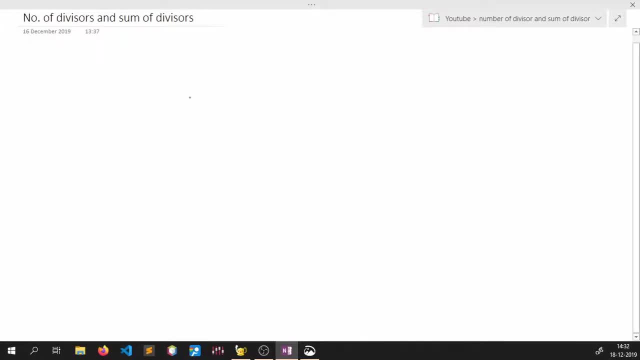 this code. now let's move on the second one, that is sum of divisors. let me clear this up. and yeah, sum of divisors. so suppose again, we have a number n which only has one prime factor. that means the number itself is a prime, or maybe it has one prime factor. so 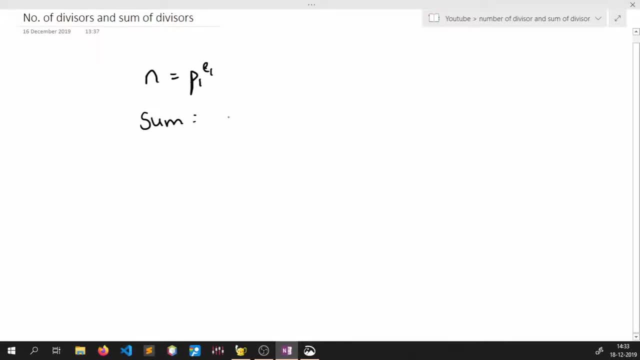 how we are representing the sum formula is that we are writing for this p1 to the power e1. we can write the sum as 1 because 1 is a factor plus p1, plus p1 square and up till plus p1 to the power. 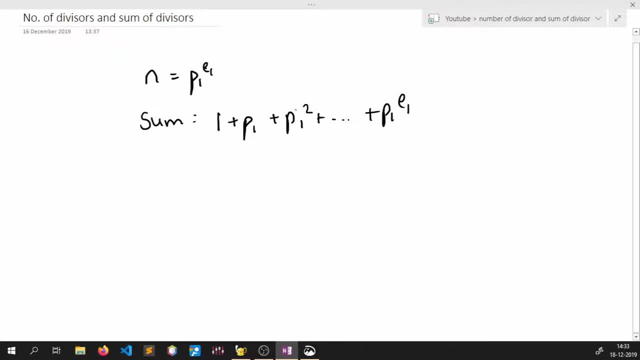 e1. okay. so this makes sense because we are adding all those factors. now this itself is: you can see, so we can write it with the sum of gp formula, which is p1 to the power e1 plus 1 minus 1, by p1 minus 1, okay, a to the power r minus 1 over a minus 1. 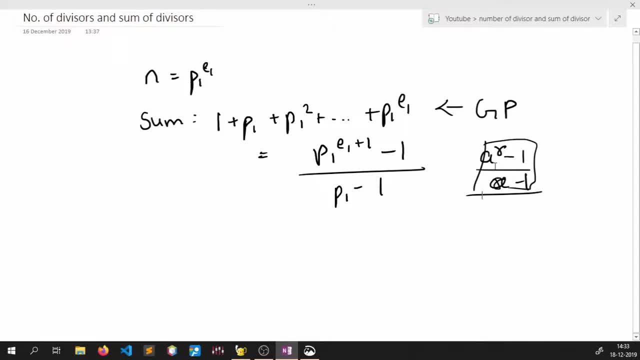 this is our formula, so let's look at this now. so suppose that this was for this form: n equal to p to the power e1, only one prime factor. what if we have to, let's look for 2. and equal to p1 to the power e1 and p2. 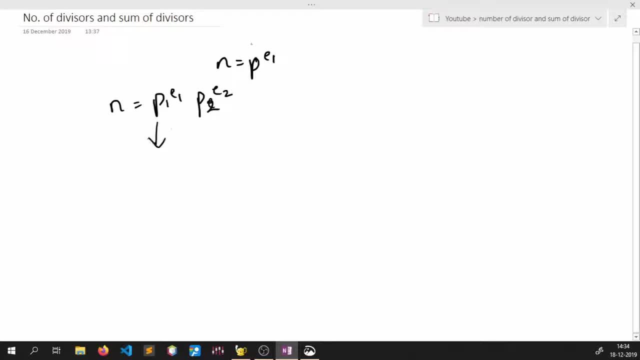 to the power e2. okay, so for this we will write the formula which we wrote for this. let me write it up for you. so it was p1 to the power e1 plus 1 minus 1 over p1 minus 1, and we are. we will do a multiplication of both of these, because we are again. 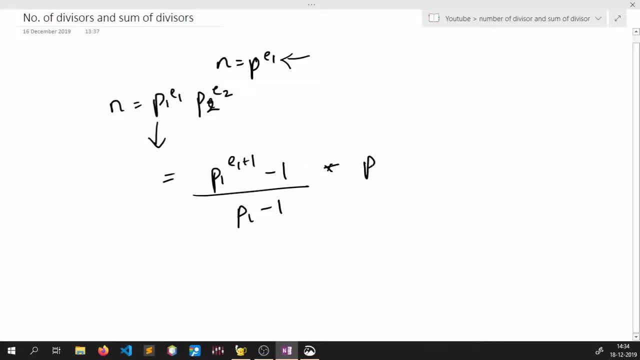 taking combination, so p2 to the power, e2 plus 1 minus 1 over p2 minus 1. so we'll write: this will become our sum formula when we have two prime factors. two prime factors, okay, and we can generalize this formula by adding a dot dot dot in. 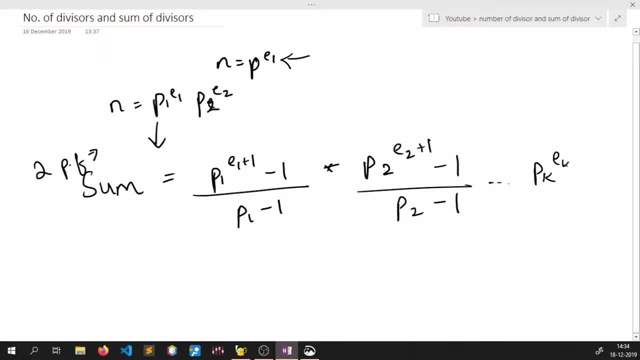 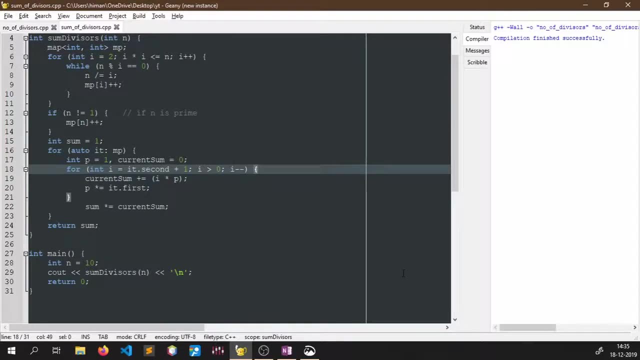 this thing, only that we'll write pk to the power, ek plus 1 minus 1 over pk minus 1. okay, so this is the formula. now let us see how we can represent this in code itself. let me bring up the code editor. okay, so sum of divisor is this one. let me take a. 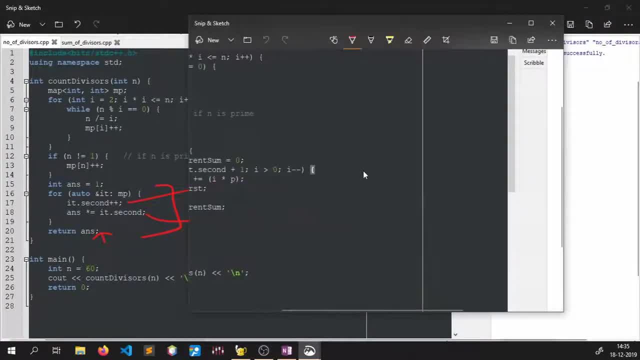 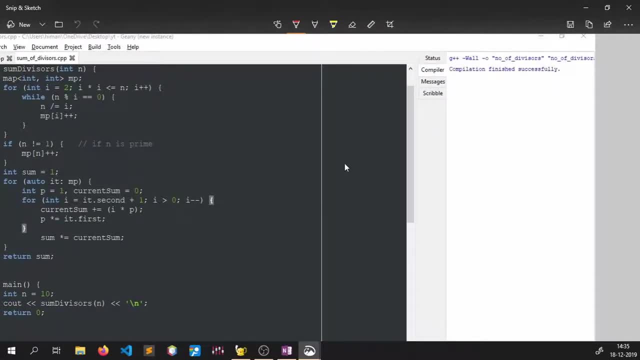 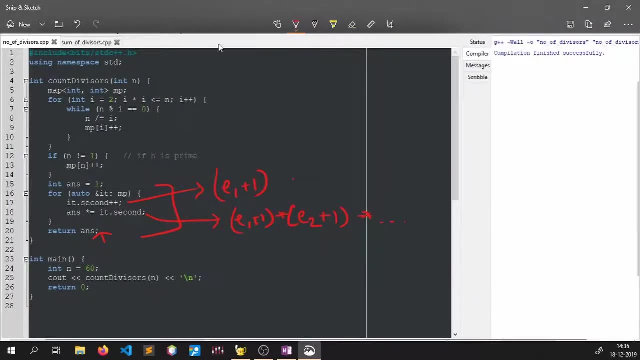 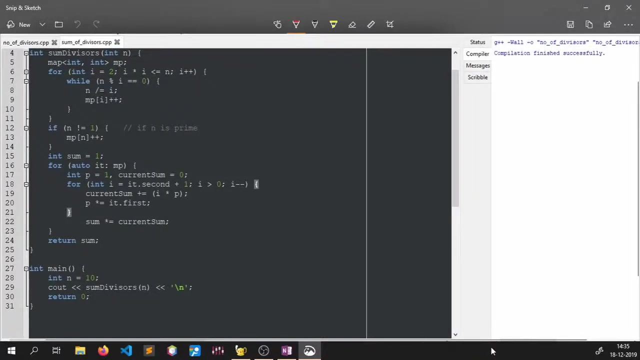 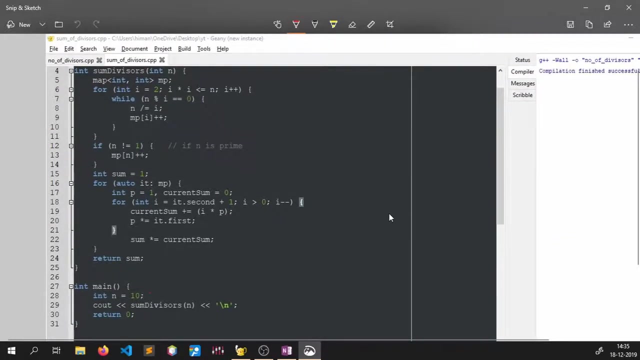 snip of this. okay, so this one. yeah, okay, this one will work. so again we have our number. there is some problem with this thing. let me correct it. okay, okay, all right, we are all good, good, okay. so again we have as example, we have 10, then we call this: 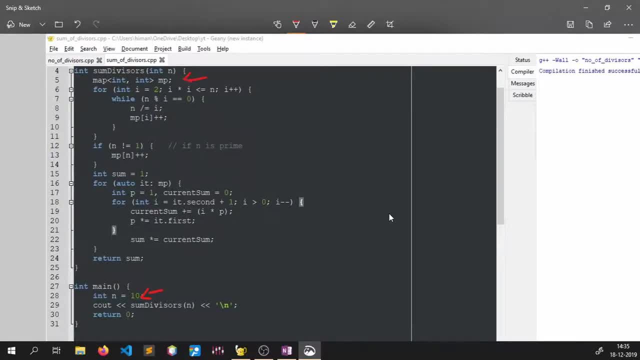 function, sum of divisor. and we go here again. we have created a map for storing the key value pair, that is, the number itself, the prime number, prime number- and its count, that is p to the power, p1 to the power- e1 form. okay, so this is what we are storing. so this localization is going to be. 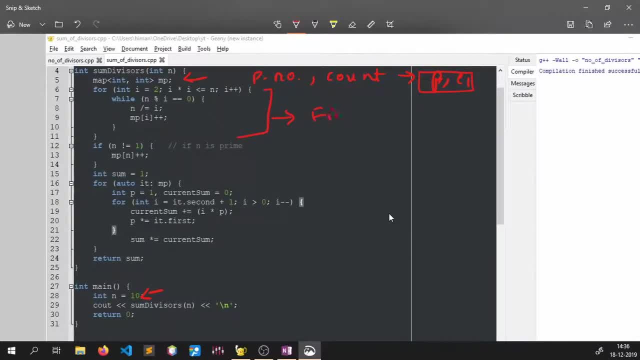 is statist and we are going to adding at the time of deepening, so we are not storing a life. it will be our new world like this: okay, and that is all we need. we are going to end this experiment, okay, and and now here we die. so we need to find a value. 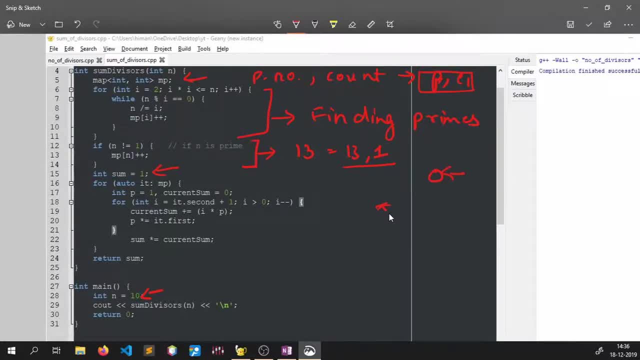 in this case, zero, then what it would simply do is it would make the whole sum as zero. so we don't want that. that's why we are taking it as one. now let's look at this one, this loop. so this loop right here is the important one. so we are iterating on the 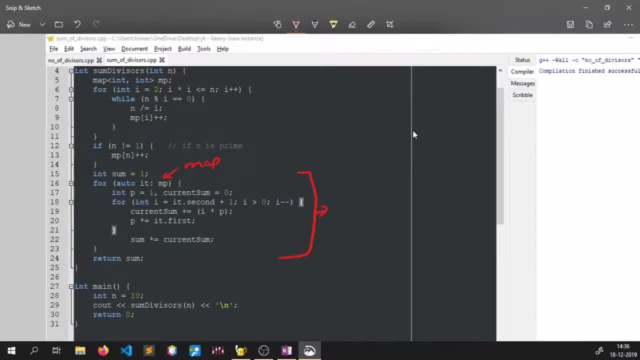 map. so this is a trading on the map. we are taking one P and one current sum. let us look why we are taking this. so we have another loop inside it. what we are doing is we are doing I equal to I, T dot second plus 1 and I greater than 0 and I. 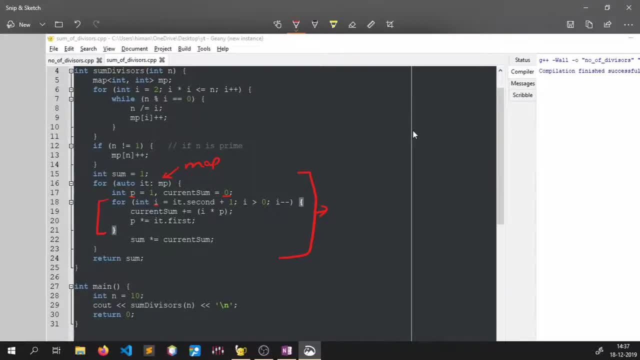 minus minus. then we take current sum, we find the current sum as I I into P, that is- let's take that thing- and equal to P 1 to the power. even so, this had a formula as P 1 to the power, e 1 plus 1 minus 1 over P 1 minus 1. so what we are seeing is: 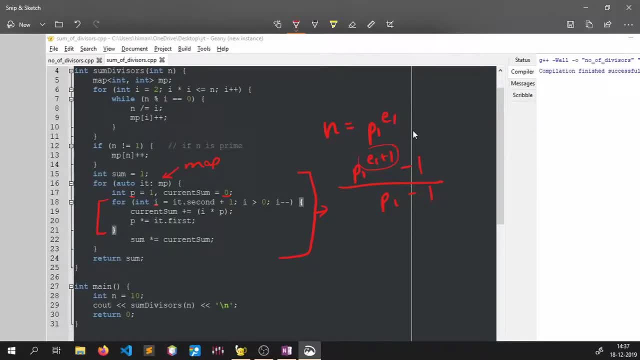 there this thing: e 1 plus 1. this is represented as I T dot second plus 1, right, and why we are not writing equal to 0. there is a reason for this. so suppose if we take this thing for e equal, e 1 equal to 0, let's say e 1 equal. 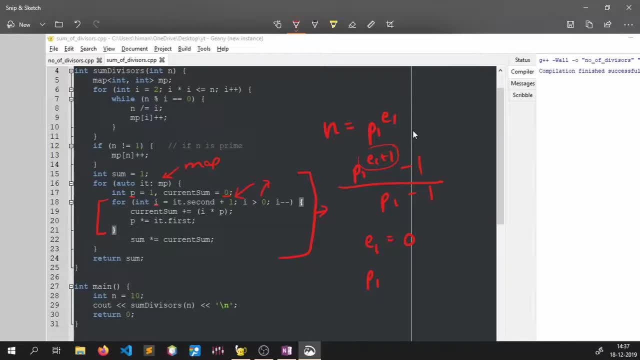 to 0. what we are going to do is we are going to take this thing and we are going to write it as e 1 equal to 0. so what will we get? we'll get P 1 even is 0, so will get 1 minus 1, and then P 1 minus 1. so this is what we, what we are getting. so 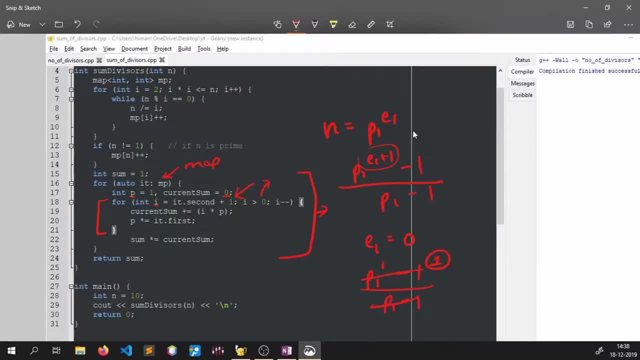 I will simply cancel out and we will get a 1 right. so that's why we did not need to take I equal to 0. we are going till I equal to 1. okay, so I t plus second. this will represent this thing, this I T plus second, and then we are subtracting it and 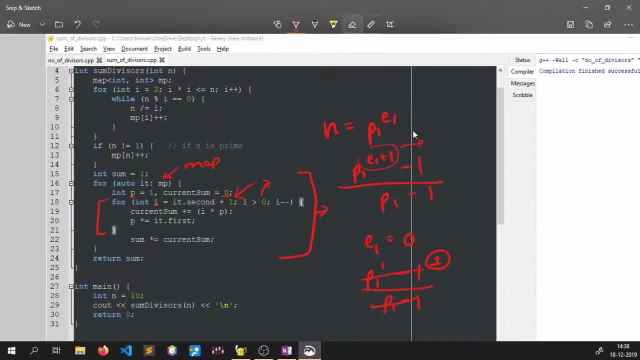 mean for this current prime. what current sum represent is for the current prime, what is the sum? so current prime, let me write here current prime. so what is the sum of that, what it is representing? right? so we have it there and then p. we will multiply it with id dot. first, why we.